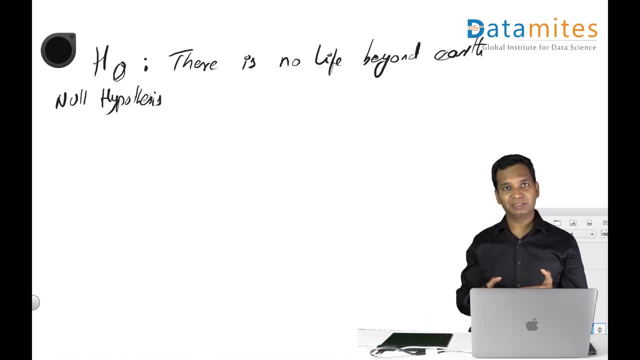 And this is a kind of assumption Or a statement we start with And your entire research is to disprove it. Or if you fail to disprove, then the statement stands Okay. And when you have a null hypothesis, we also have. 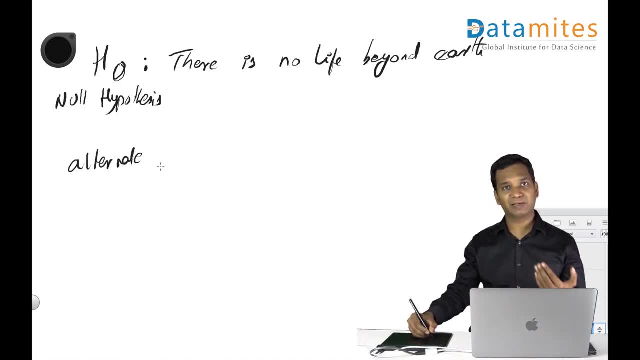 alternate hypothesis. You can have several alternate hypothesis. For the scope of this video, I'm only considering one alternate hypothesis, which I say H, alpha or HA, And that is opposite of what is null hypothesis. There is life. There is no life beyond Earth. Okay, So this is called a setting up your hypothesis Before you want to do any research. 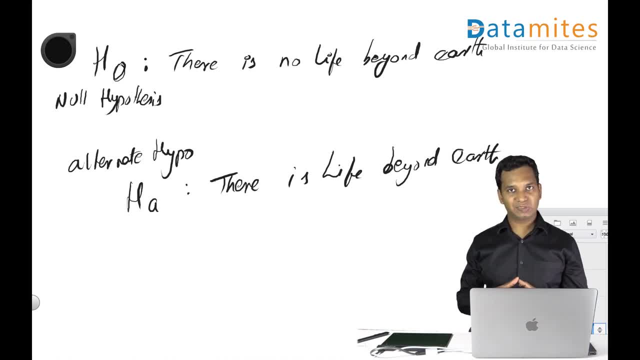 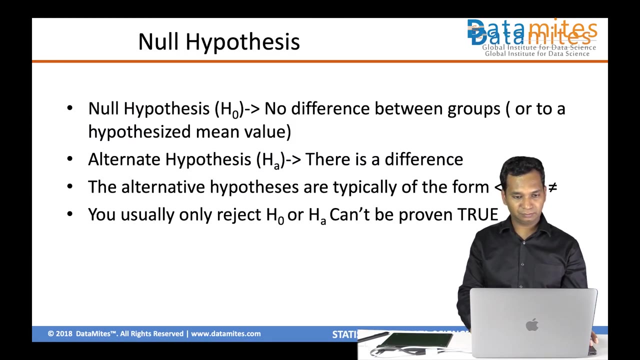 or prove or disprove phenomena. we set up the hypothesis, In our case H null is there is no life beyond Earth And H alternative is there is life beyond Earth. Alternative is always opposite to the null hypothesis. We'll get back to the slide and see what they have. Okay, They're explaining that. 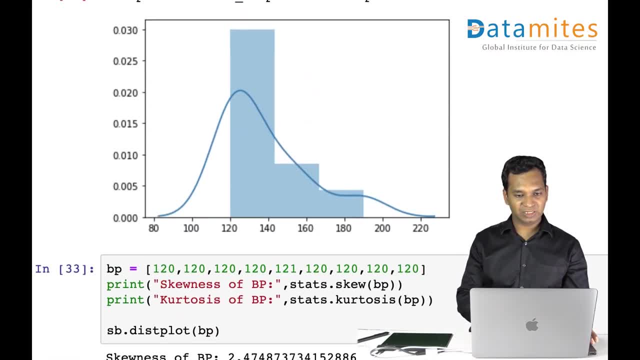 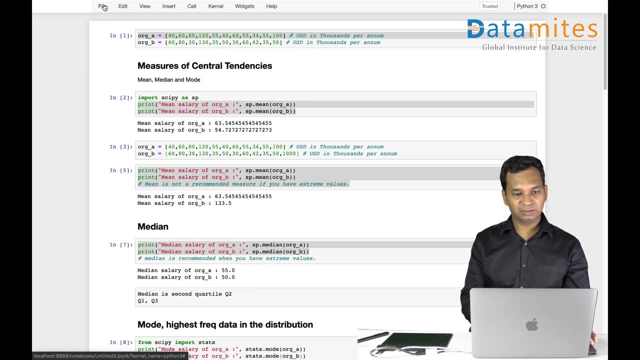 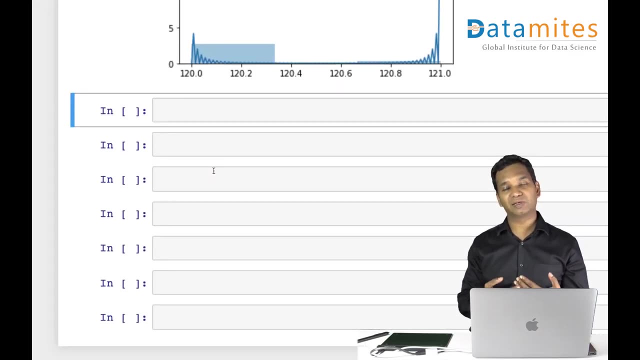 And this is the previous one, all of your. So I will leave this code in the description itself so that you can download and practice it by yourself. So I'm going to continue in the same sheet. So I call this as hypothesis testing. Okay, 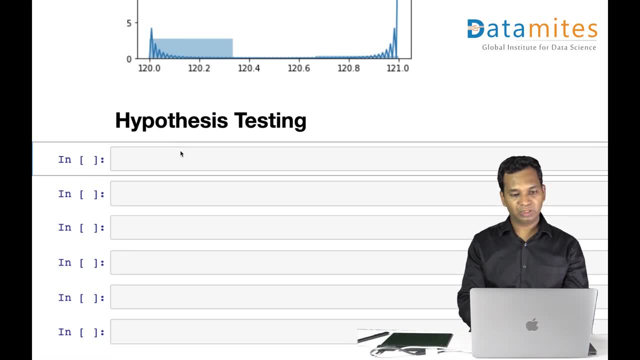 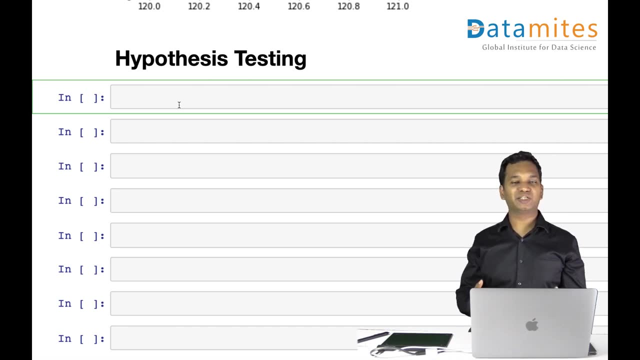 Alright, Okay, Okay, Okay, Okay, Okay, and i'm going to take a simple example to to explain you what is hypothesis testing. so let's take average marriage age, okay. so in india, the average marriage age was about 27- 28. now it's. 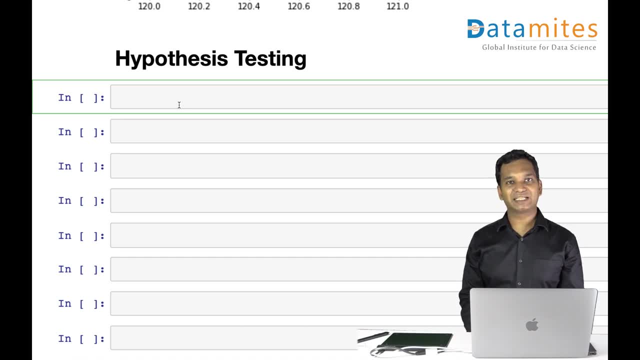 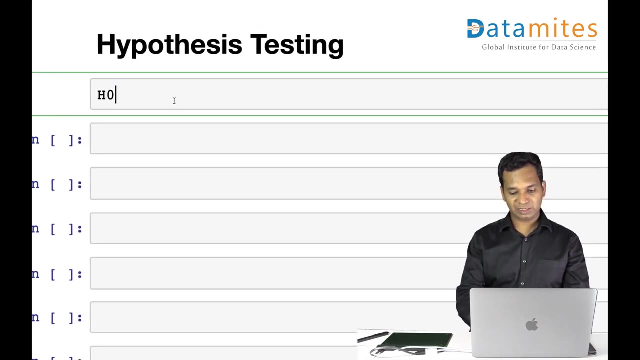 shifting towards 30. it's about 30 now. so i want to statistically prove or disprove. in this case i want to prove that the marriage age is 30. so i'll start with a null hypothesis. my null hypothesis is marriage age. so i should be very specific: whose marriage age? so i would say marriage age of 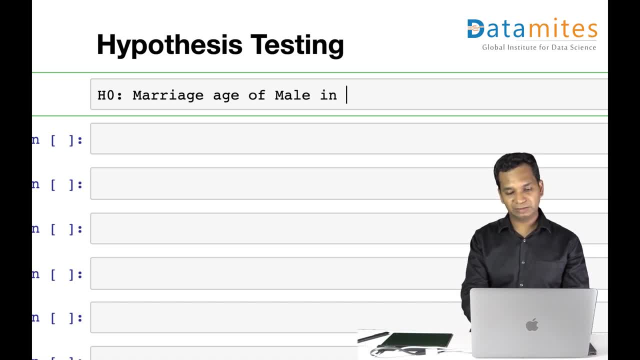 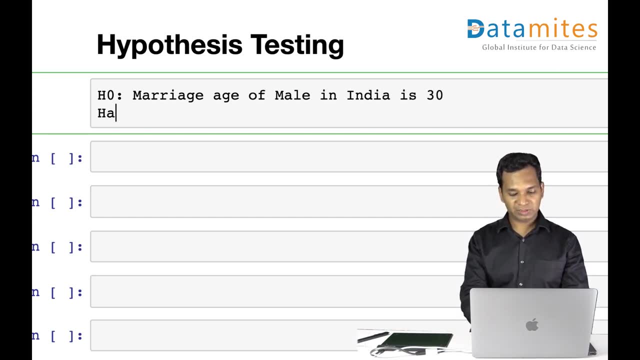 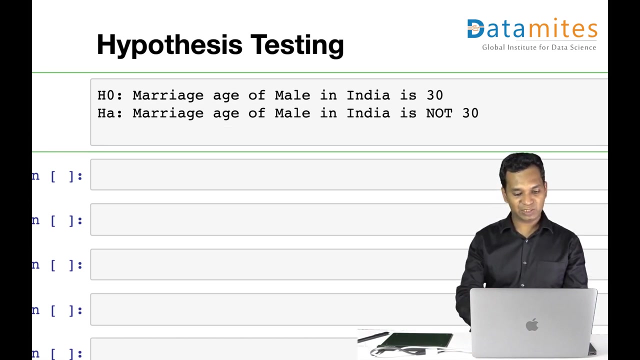 male in in in india. so is 30. my alternate hypothesis automatically will become: marriage age of male in india is not 30, so this becomes my hypothesis setup. okay, so you could observe that. okay, the 30 is actually called as hypothesized mean 30 here. 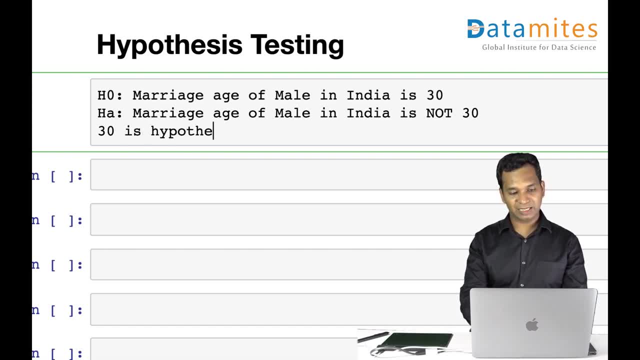 30 is hypothesized mean in this case, in this research. so what is 30? this is what i want to prove. i want to prove or disprove that 30 is a marriage age of a male in india, okay, and 30 is called as hypothesized mean or an assumed mean, which i want to compare. the distribution you can. 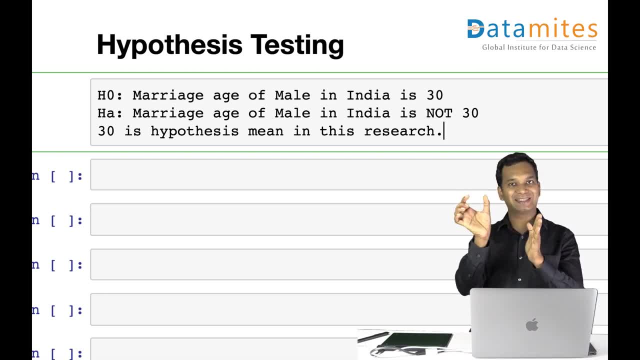 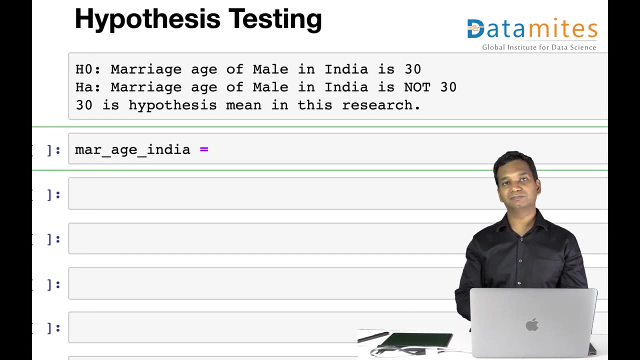 see that null hypothesis is comparing a distribution to a single value is comparing it. in this case it is 30. so i'm going to say marriage age in india is equal to well, ideally, you need to collect this data from different channels. one of the best channels to collect this data is facebook or any social media. so facebook, you can simply. 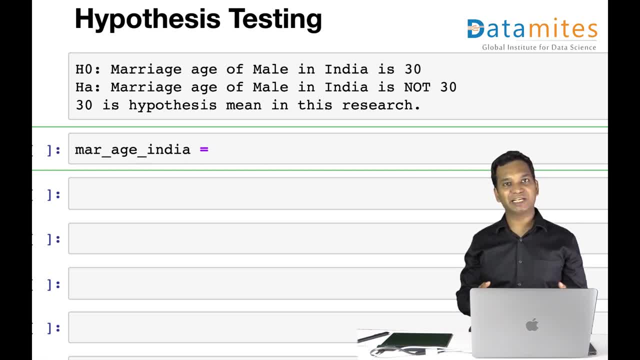 run a poll saying what is a marriage age, what, which, what age you got married. so you have to actually take a sampling from married male because this only applicable is a marriage age. so when did you get married? so it's only married people in india. you basically put the filtering in in facebook poll saying india male unmarried. 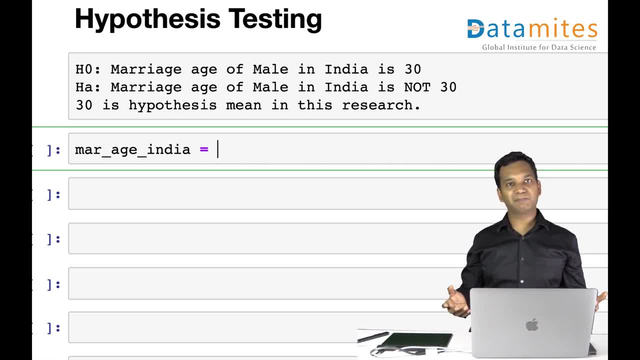 accordingly, it will show to the only people and it will be, of course, random sample, because facebook shows that many different people. and well, if, hoping that everyone is using facebook nowadays it is more or less true, so we could take that as a broad india population. okay, and marriage age: uh, after the survey is done, of course, you need to incentivize the survey. so if 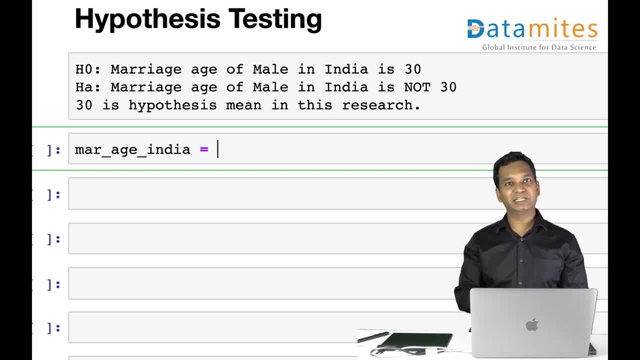 you want to do it. you say that now give me your marriage age- uh, anonymous, of course, and you will be getting a pdf or document or a book, video book which says how to live a happy married life. and, trust me, people always fall for that and they might take your survey. so, um, i'm just gonna guess. 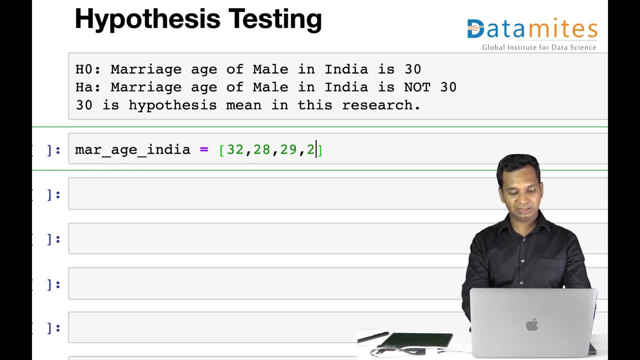 a 32, Uh, 28, 29, 31, um okay, 29, 31, 34, 33, 32, 35, 35 again, so 32. Okay. so you know you might get 1000 2000 uh data. so i'm just taking few data for explaining the things, all right. so this is. cứ wollen giamt назв� ansếu. ann segundos: the marriage age of uh india, which is UK and India in that age, meet and sign language and document. like, how would you do that? right? of course i would say yes, because obviously you want to study. let's just review lunch with you and make a small review, so i might, as 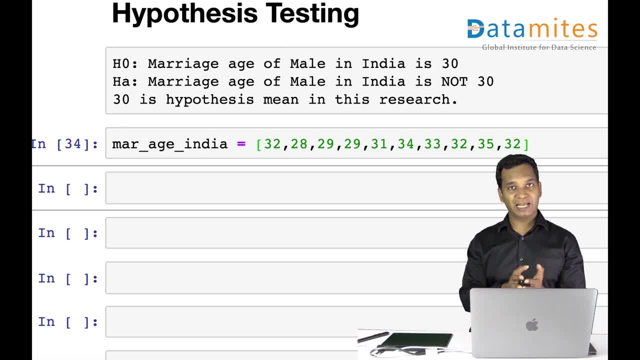 which supposedly you got from Facebook: random selection, random sampling, And let's say it is thousand records. I have only a few here. So in hypothesis testing- so there are different tests For this- we should be going for what we call it as. 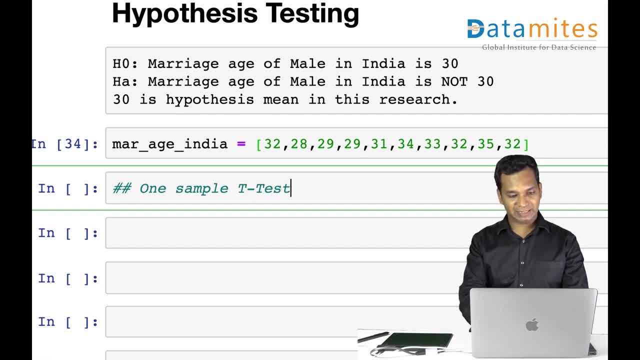 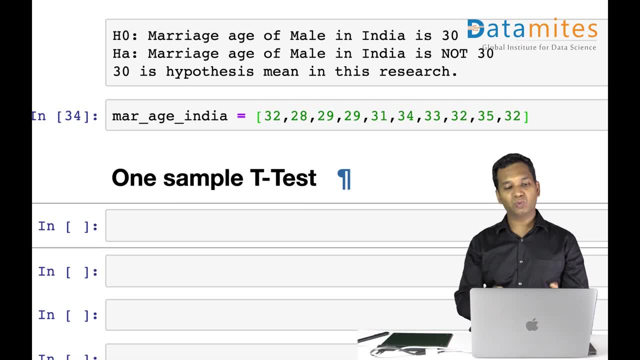 one sample t test. One sample t test. One sample t test. In one sample t test we compare one sample distribution, which is a marriage age here, with a hypothesized mean which is 30, okay, So how do you do that? 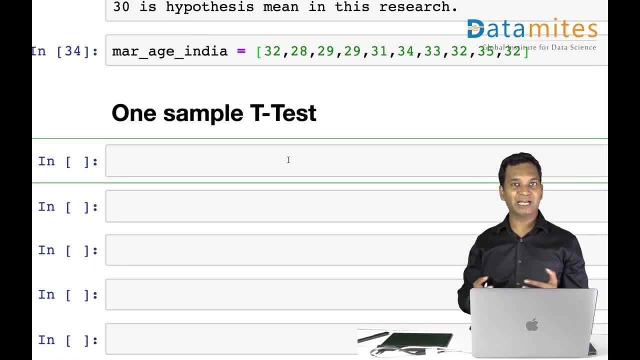 Well, we have t test, a module which is actually a statistical module. We can also do it manually. We have t formula- I'll explain that as well- But we have Python stats, so we can simply say statsttest. one sample: 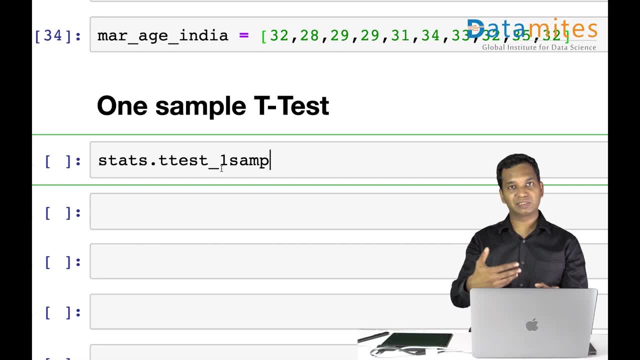 So by pressing a tab, you can retrieve all the functions or modules in Jupyter. So I'm just that's what I'm doing. So this is one. If you're trying to copy from my video, just make sure that this is not L, this is one. 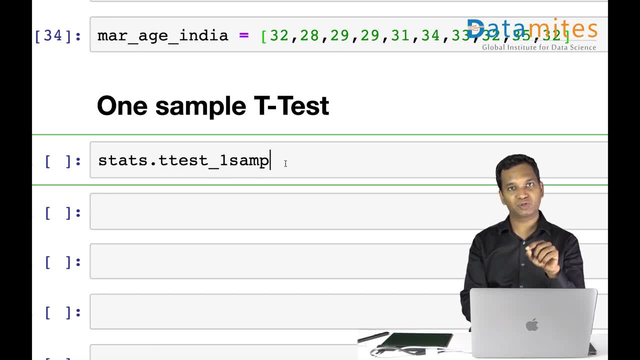 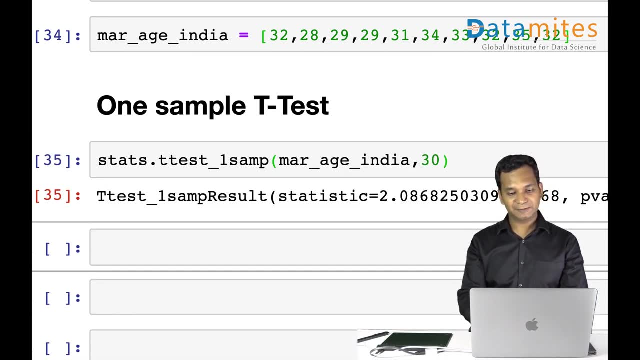 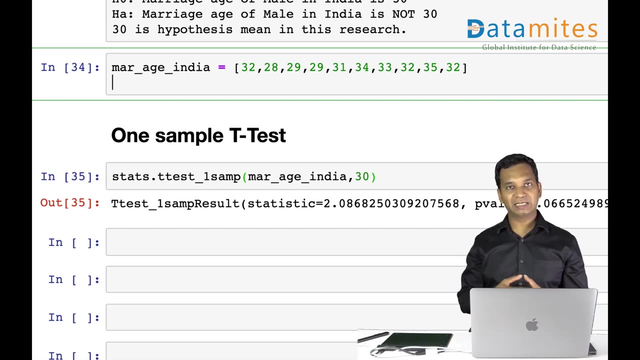 Most people make that mistake. It's one sample. t test underscore one sample. I'm gonna pass my marriage age India and then pass 30 hypothesis mean Run this All right. so just before doing that, the t test and whatever test I'm talking about, you know. 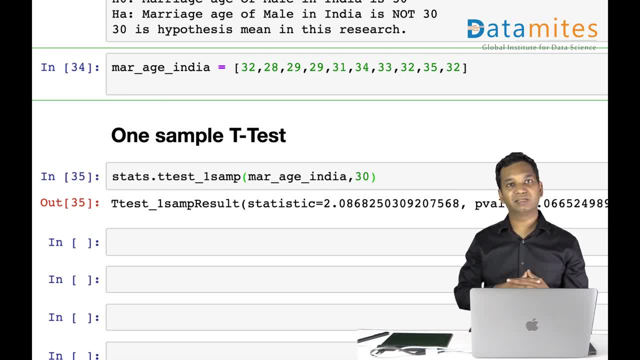 what is analysis of variance? is parametric hypothesis testing methods. When you say parametric, we have to ensure that the data is normal. If the data is not normal, we cannot use the t tests. So first of all we need to print. 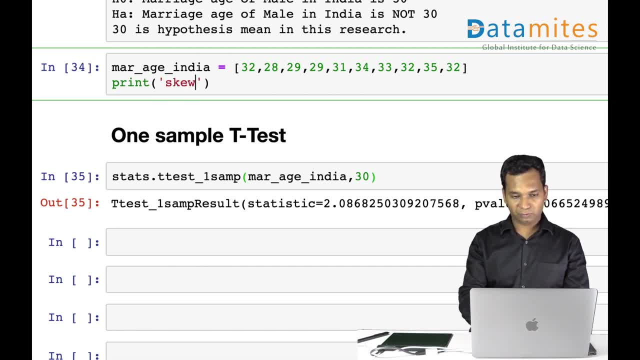 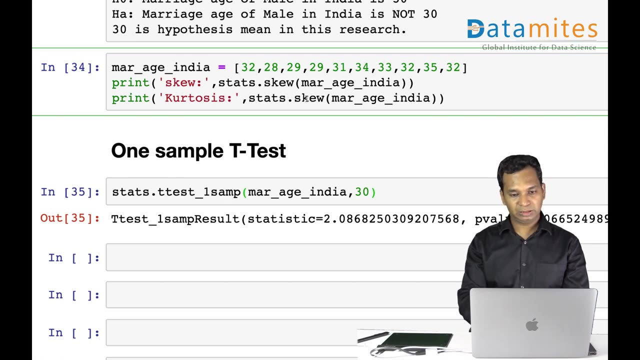 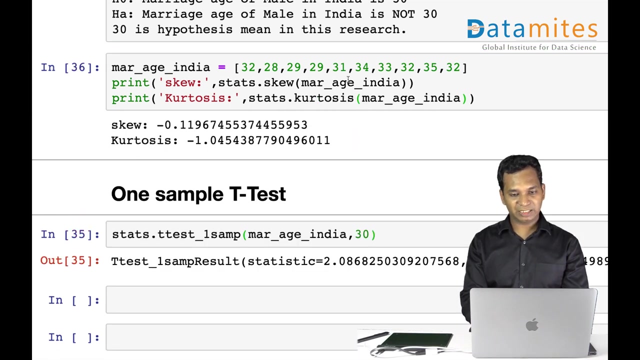 let's say skewness of the data and the kurtosis all right. So let's say statsskew and marriage age in India: Okay, copy this and say kurtosis. and say, oh okay, Kurtosis and oh okay, slightly more kurtosis. 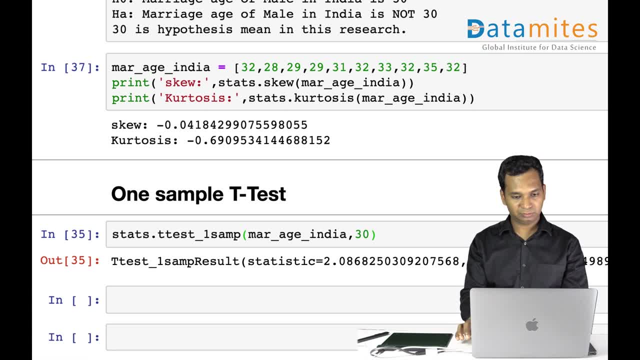 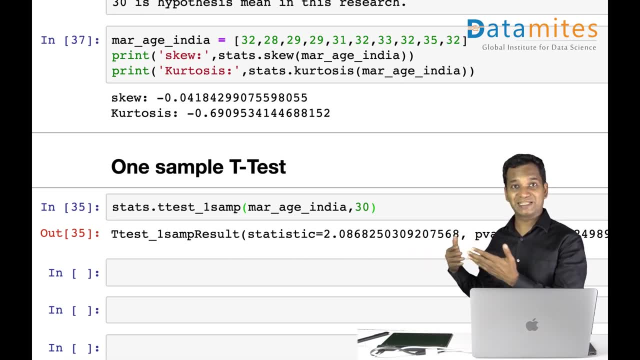 So I'm gonna reduce this to 32, maybe. Okay, now it's okay. So I have a skewness which is almost near to zero. It's 0.04, which is wonderful. So your data distribution is perfectly symmetry, okay. 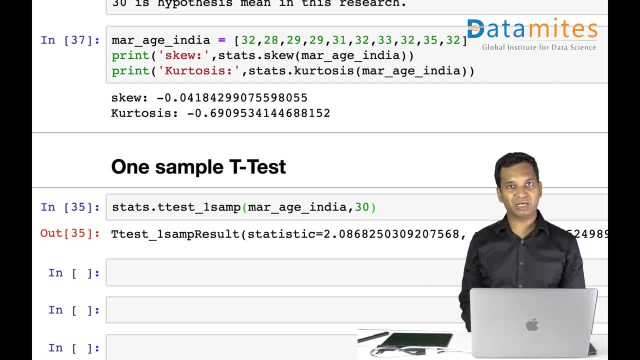 Like perfectly symmetric Skewness is also less than minus one, So it is little flatter. I can see that most of the data is around 30. So I'm gonna make it little, not flatter. There's a guy who married at 25, poor guy. 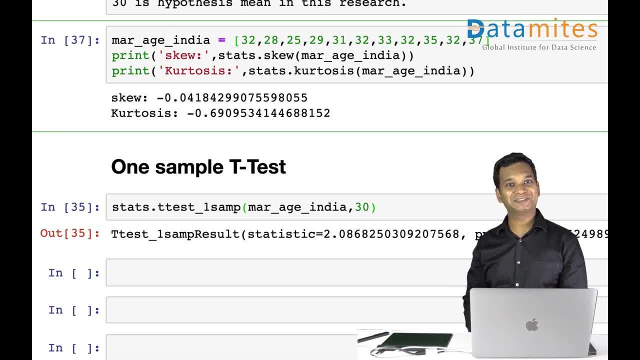 and 37, lucky, isn't it? Marrying late is lucky. you have a lot of time for yourself. Okay, let me see Now. your skewness got little towards the negative side and kurtosis is perfectly Zero, which means you have a perfect distribution. 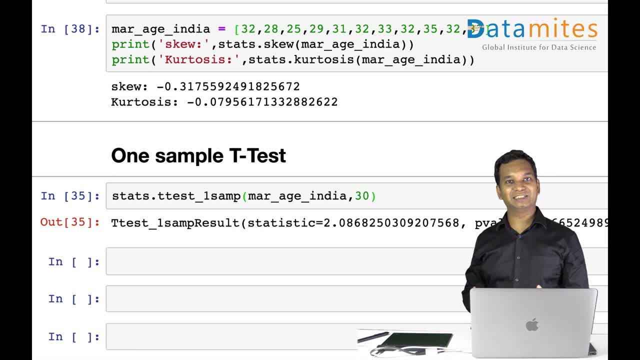 Okay, you know, in general terms, you cannot tweak the data. In fact, if you take the data, your research becomes invalid. Whatever data you get, you can of course remove the outliers, but other data you cannot remove certain part. 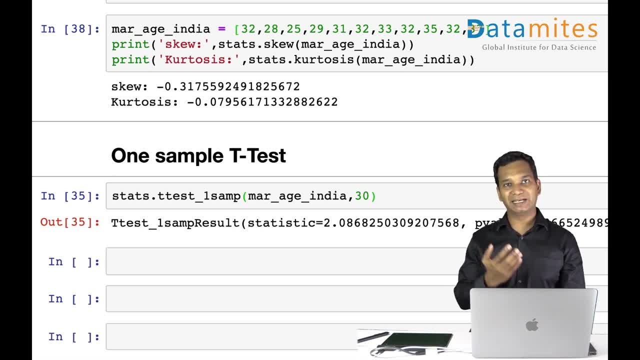 then it doesn't become a random sample. So you should be retaining all of your data which comes from the survey, just by removing the outliers. So if you do a tweaking like what I'm doing, your research becomes invalid. Okay, Okay. 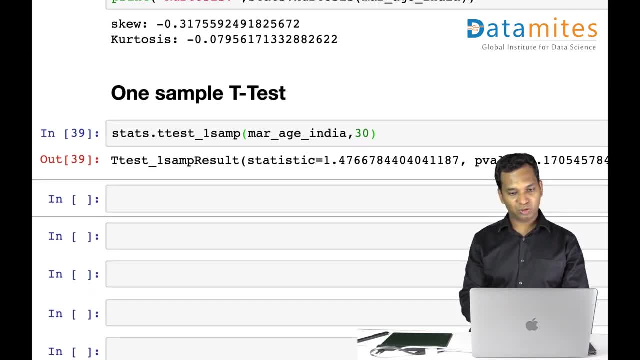 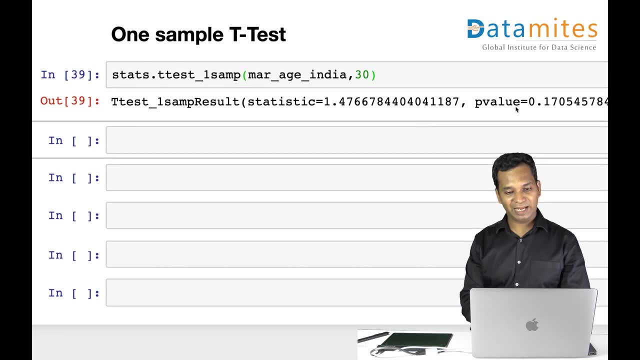 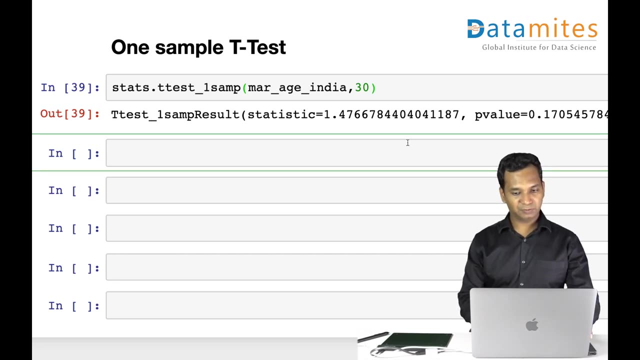 Okay, so now I run the same test again. So from my test I have two values: One is statistic, Another one is p-value. Okay, Statistic and p-value. P-value is nothing but probability value. So it's my test, is my t-test is telling me: 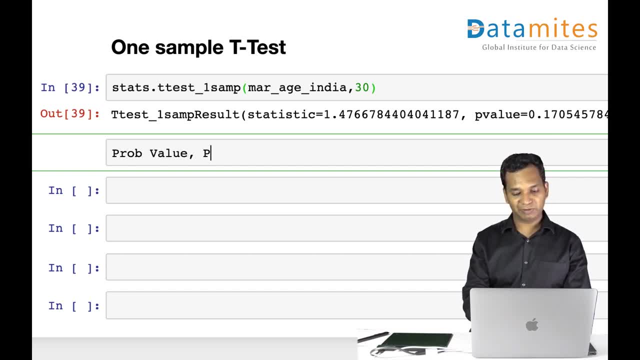 that probability value or p-value- simply p-value- is equal to 17% Or 0.17, it's like 17.05%. So which means that there is 17% chance that 30 is a marriage age- 17% probability. 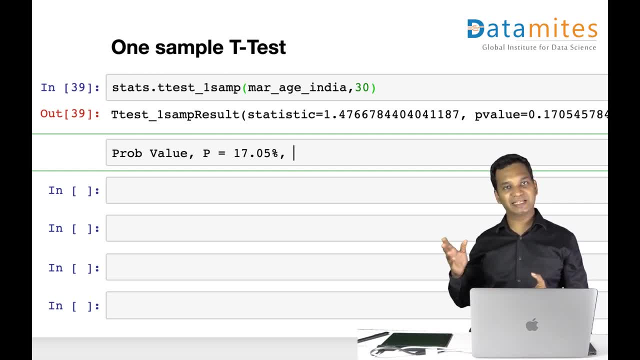 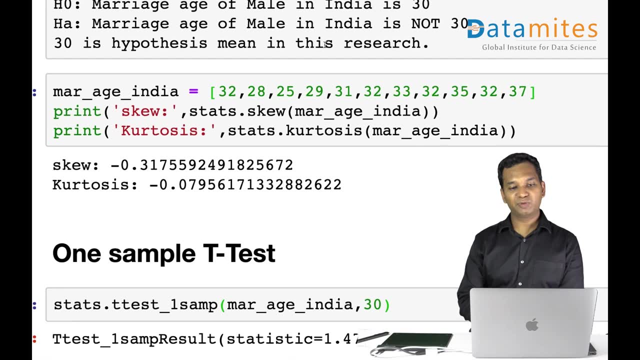 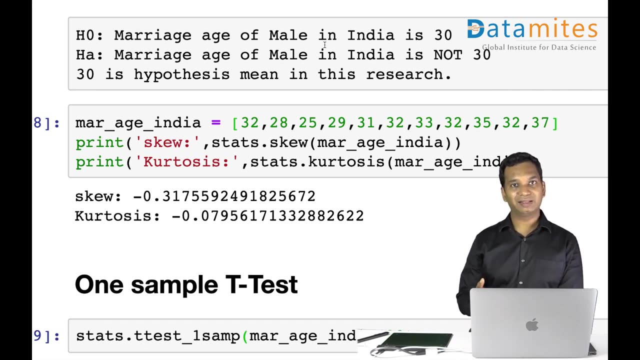 or chance that the 30 is a marriage age of your distribution. Now the question is: with this data, will you be able to reject the null hypothesis or accept the null hypothesis? Yes, If we reject the null hypothesis, then we accept alternative. 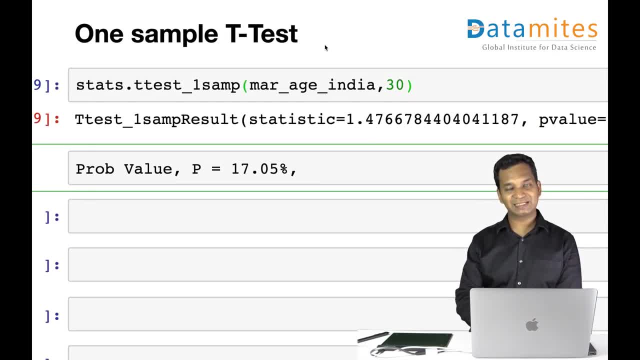 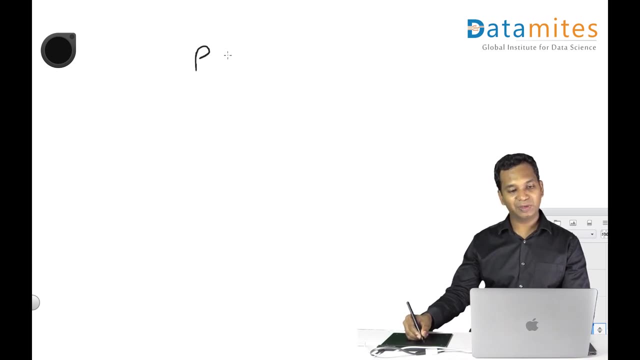 So null hypothesis says marriage age is 30. My test says there is 17% chance that 30 is your marriage age. Okay, Here you need to know something As a thumb rule you can remember if the p-value is less than 5%. 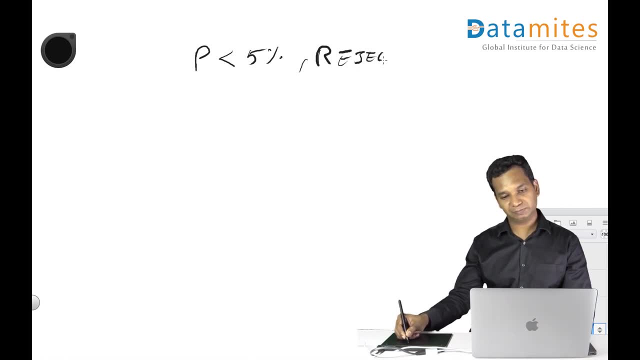 then we reject null hypothesis And this is kind of really, really thumb rule for you. you can remember it, And this is 95% confidence interval study. This is very common for most of the research, but if you're doing something related to medical or food, 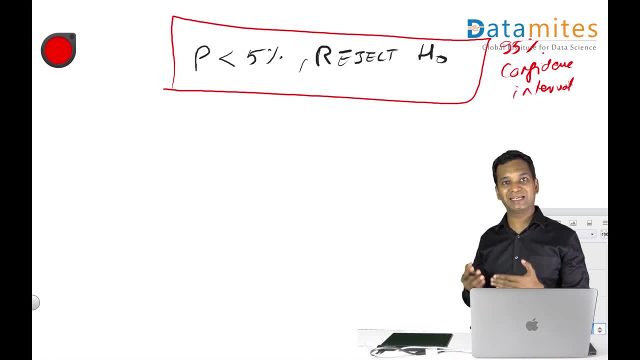 you might go for 99% confidence interval study where the p-value has to be less than 1% to reject the null hypothesis. But for you, for most of the statistics purpose, a data science purpose- p-value less than 5%. 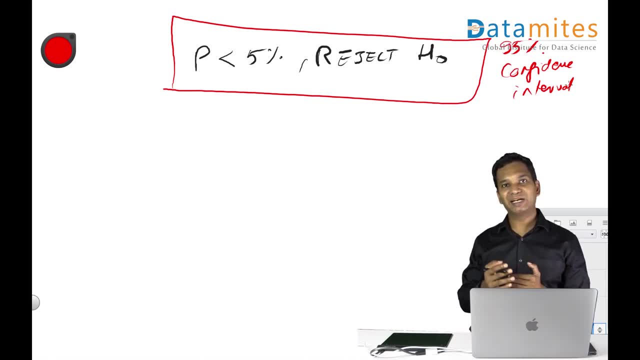 you can reject the null hypothesis, which literally means: if the problem is, you can reject the null hypothesis, which literally means: if the problem is, you can reject the null hypothesis, which literally means: if the problem is, the probability value is less than 5%. 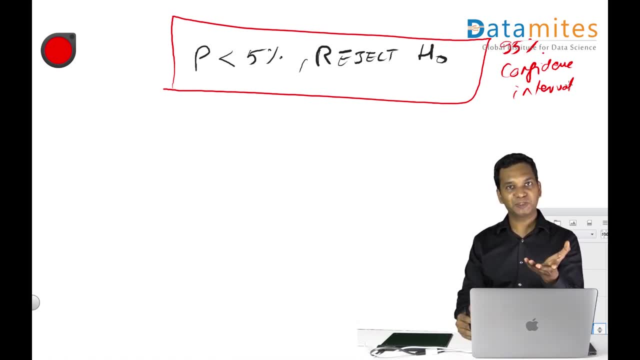 If there's less than 5% chance that 30 is a marriage age, then you can reject the null hypothesis which says that 30 is marriage age. Makes sense, isn't it? Less than 5% chance is nothing, So we can reject it with 95% confidence. 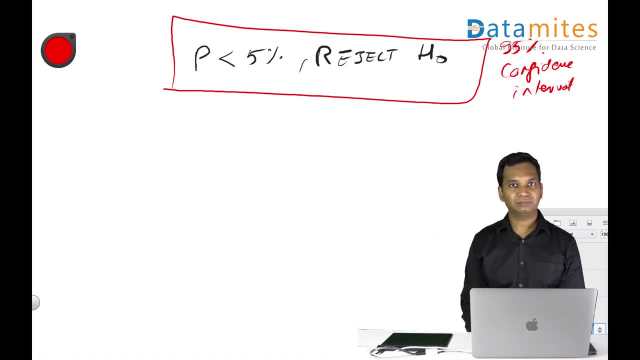 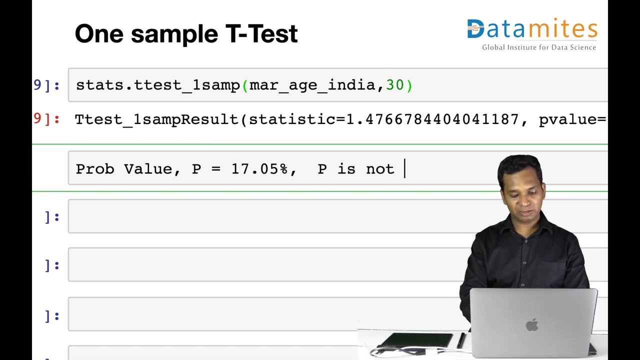 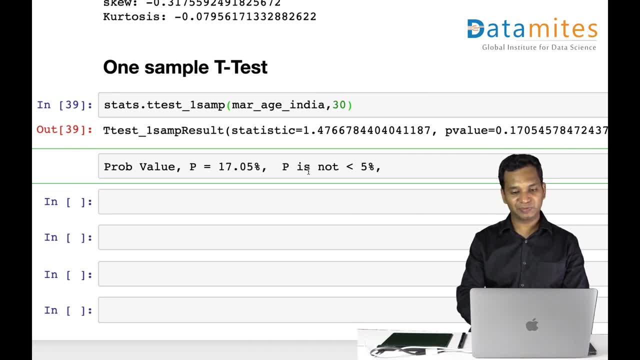 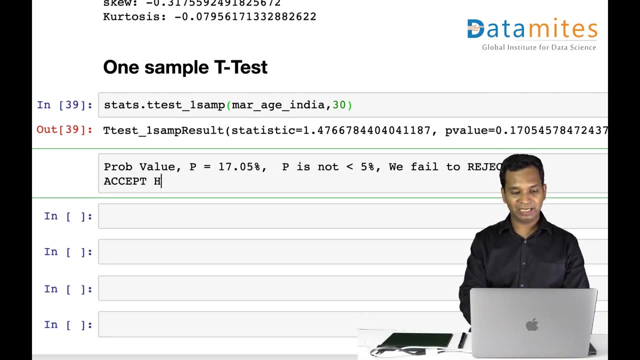 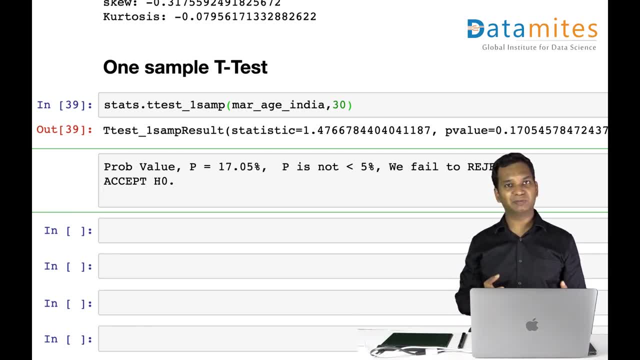 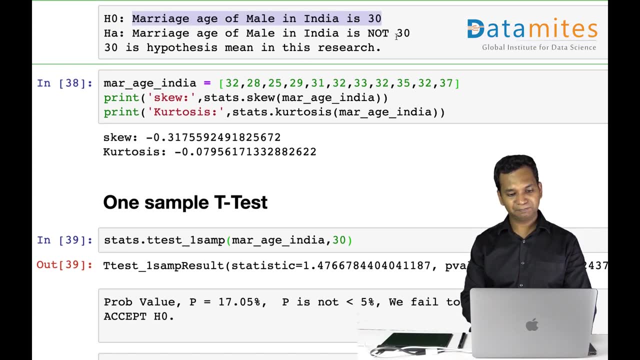 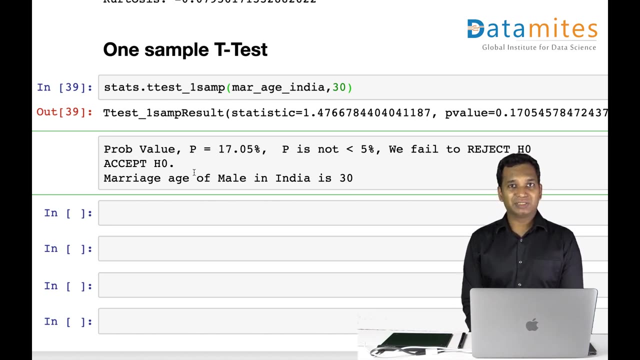 Hey, you only have 17% probability of 30 being marriage age. You gonna accept null hypothesis and say marriage age in male India is 30? Doesn't look sound like a more logical conclusion? Yes, that's true. so this is. doesn't really look nice because you have. your research is weak actually because you 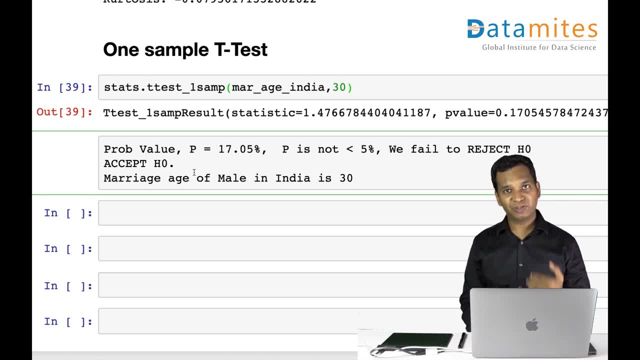 are you fail to reject the null hypothesis. if you successfully reject the null hypothesis, then you can strongly have a statement with 95 percent confidence that marriage age is not 30, which is an alternate hypothesis. because you fail to reject null hypothesis, your research itself has become weak a bit and it doesn't have a strong statement. so we cannot reject the null hypothesis. 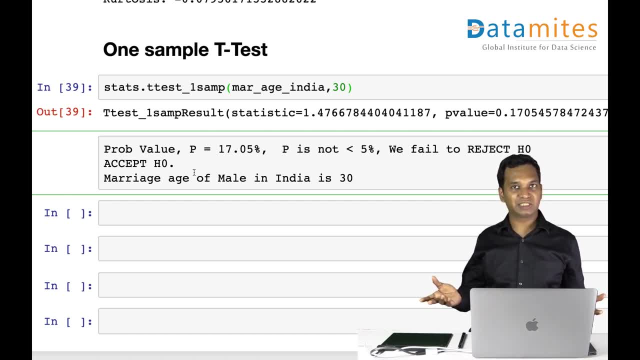 so we accept it, not happily, but that's the way the research is. so you cannot make a strong statement, hope it makes sense. okay, so this is one sample t-test and it's. it's really really powerful t-test, powerful test to, to, to demonstrate a phenomena, to prove or disprove phenomena, equating it to. 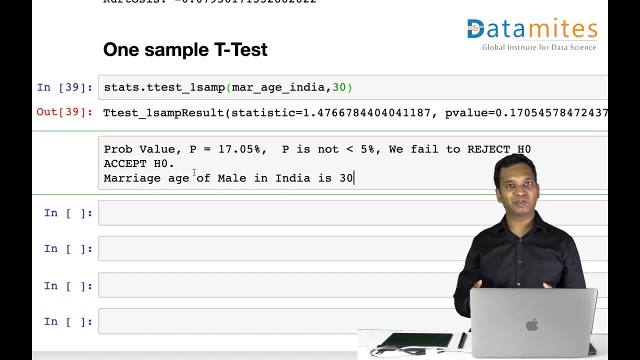 a single value, which we call it as hypothesized mean. so what i'm trying to see is say is that the 30 is not in this case, 30 is of course. you cannot reject it. so that is of course, a mean of this hypothesis, which means, yes, most of the 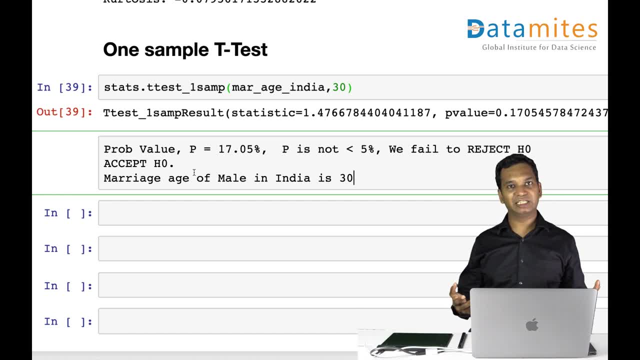 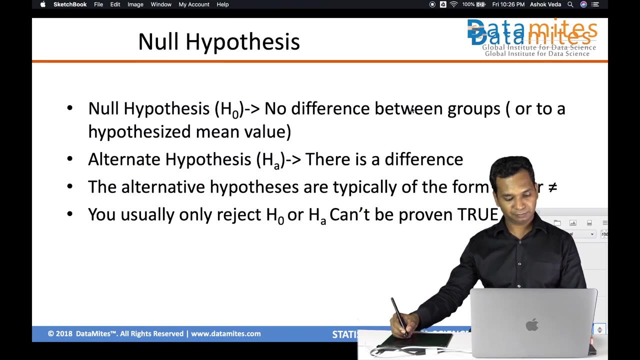 indians or indians get do, get married at 30. we cannot reject that. that is not the marriage age. we cannot reject the null hypothesis. that is marriage age. so if you look at the graphical way of doing this, what we have done here, okay, okay, all right. so. 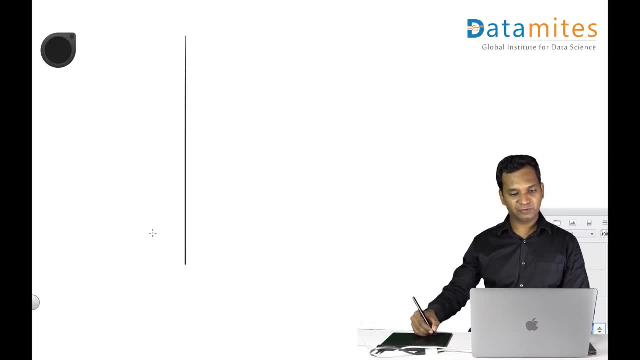 let's say you draw a histogram of all the people who have collected. let's say you've collected 4 000 people of the marriage ages and you draw a histogram and assuming that it is a nice normal distribution like this, and let's say, the phenomenon of the t is around. 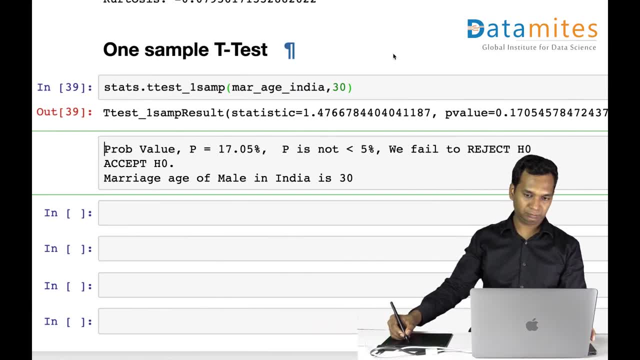 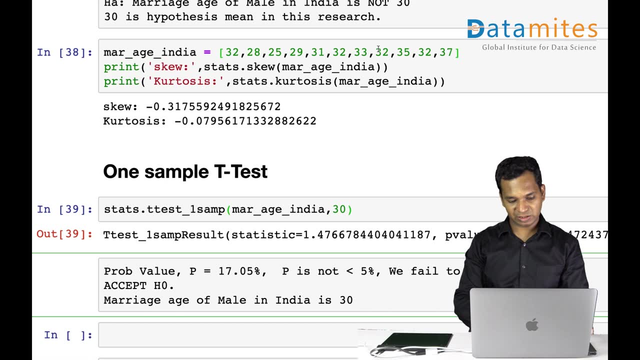 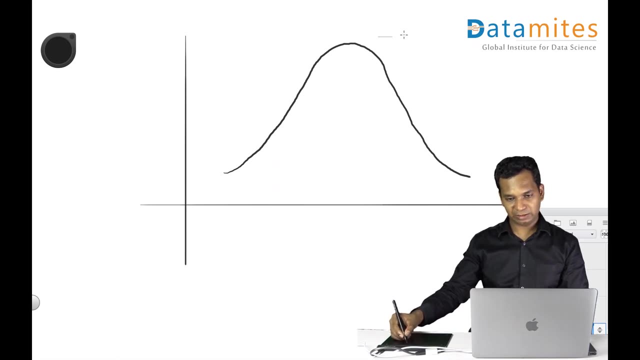 um, just saying it said that is coming. t is positive means this is greater. okay, so 30 is somewhere. let's say here, okay, and this is, this is 31, this is 32, and this is 29, and this is 28, and this is 27, and so on, so forth. okay, so, if you so, this is your entire data. so i 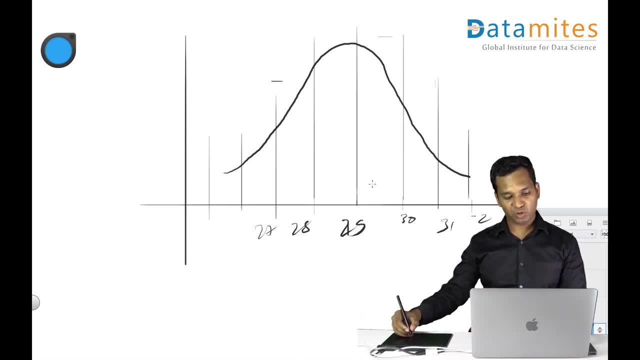 want to find the problem, so i want to find the problem, so i want to find the problem, so i want probability of 30 being my marriage age. so when you want to say 30, so 30 actually can be taken as this region which is between 29.5 and 30.5, the disc that the area between these two can be taken. 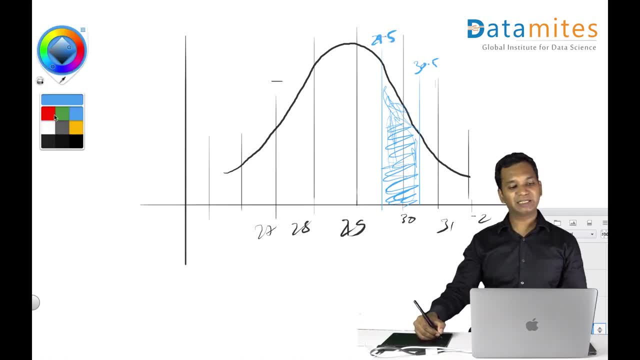 as 30. what's the probability generally? probability p is is actually desired outcome by total outcome. if you say what's the probability of getting a head in a coin toss, so you say 50 because you're looking at head as one desired outcome. total outcomes is head. 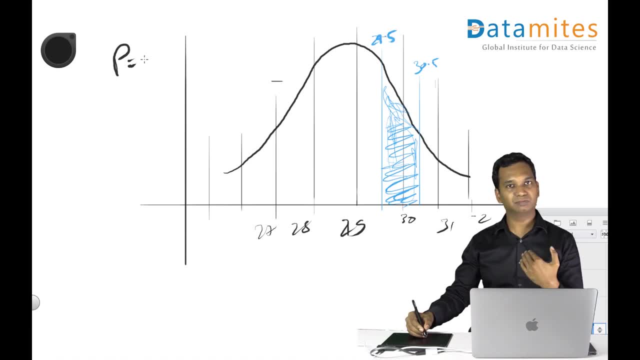 or tail, which is two one by two, is fifty percent. it's simple. so of course it's again high school mathematics. hope you remember that. so in this case, let's say: this area is what actually is: 30, representing 30 divided by total area, which is the entire area of this curve. so i'm just gonna. 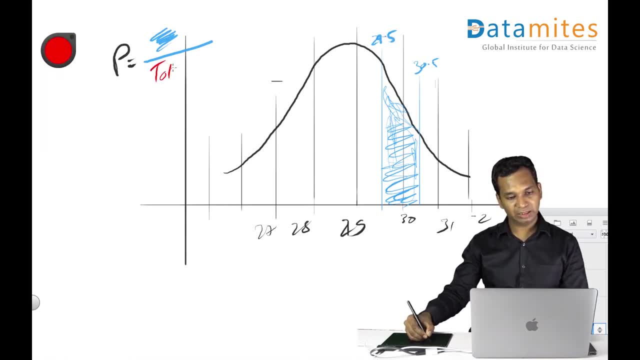 write it down with the red color, for example. so total area, which is this entire area. so we got a value of 17 percent. approx, which is representing this area, is 17 percent of the total area and that is your probability value in the t-test. so it's so easy. 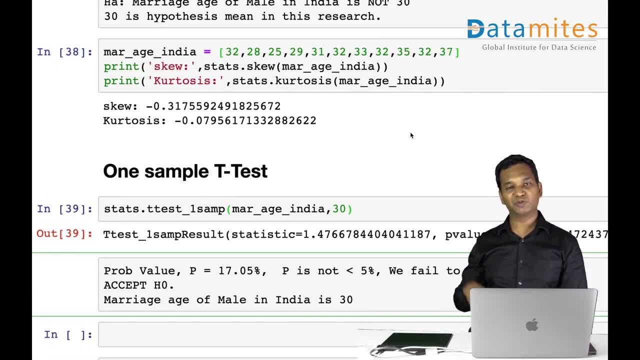 that your module t-test, one sample t-test, is giving you the probability value straight away by calculating it from the way i showed you graphically. but what if, if you don't have this kind of tools and and probability values? traditionally people used to follow t value, so the statistic given over here. 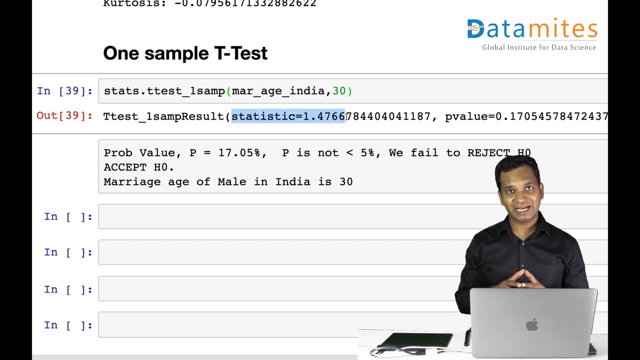 is actually a t value. as a data science scientist or data science professionals, whatever i'm going to tell right now is not really required for you, because it's very simple for you to just look at the p value. less than five percent: we reject the null hypothesis. if not, we fail to reject. 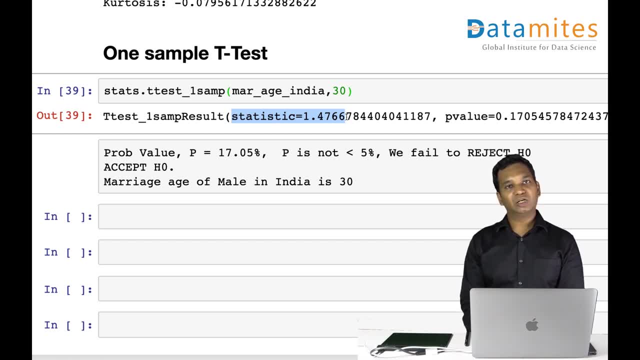 null hypothesis. so we accept null hypothesis. but just to know the background, what is the statistic? so statistics, as you know from our previous discussion, is a parameter, is is a summary of a sample variable. okay, so this is a t value actually. so t value in our case is act, is 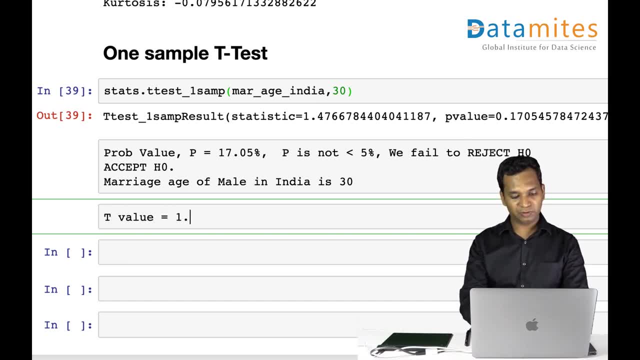 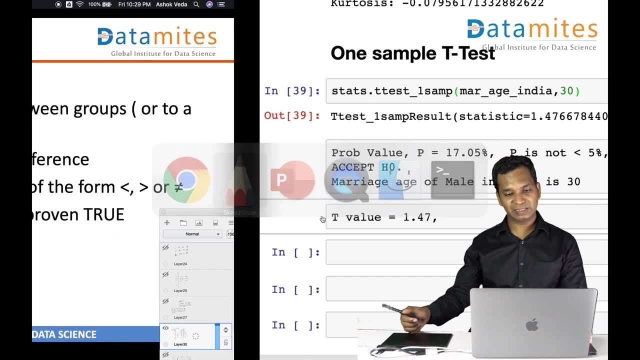 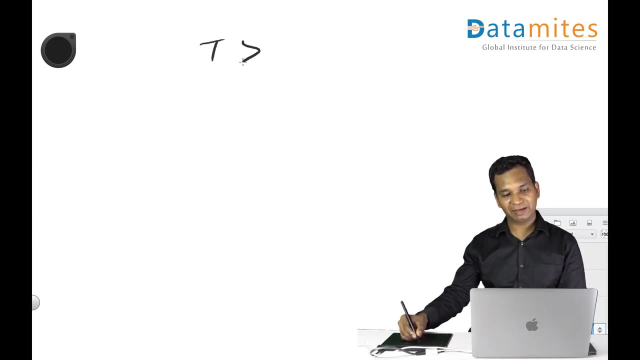 t value in our case is actually 1.47, so you could also reject a null hypothesis if the t value is okay. so if the t value is greater than t critical, we can reject null hypothesis. it is very similar to what we have discussed before if p value is less than five percent. 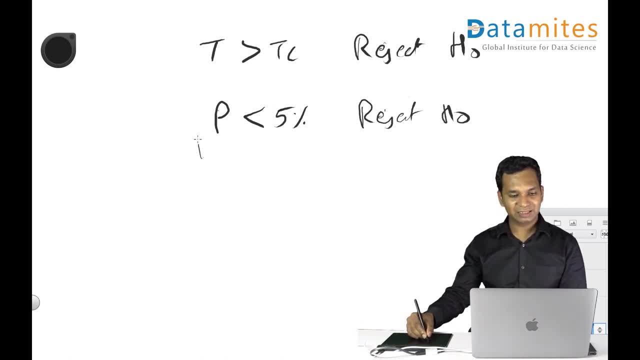 we reject null hypothesis. in this case we can simply say: less than five percent reject null hypothesis, no further questions. but here we only have t value. we need to also find t critical. how do you find t critical? well, t critical is found by looking up that table. 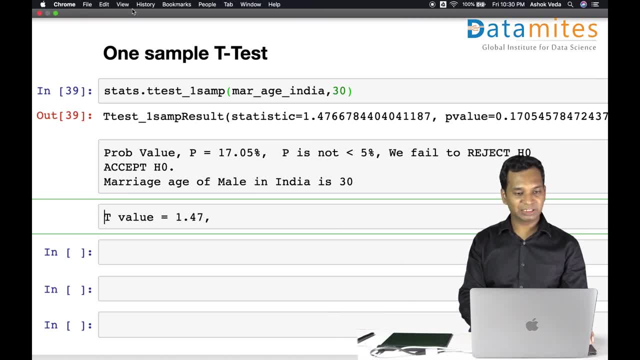 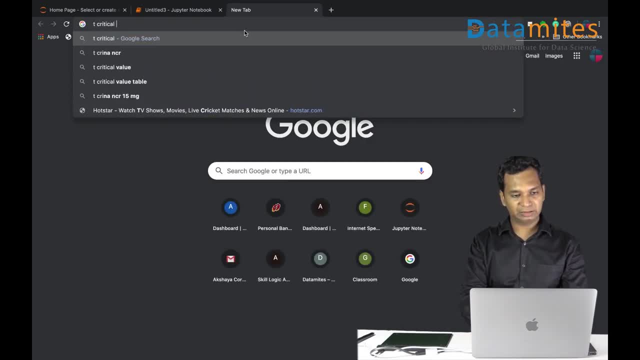 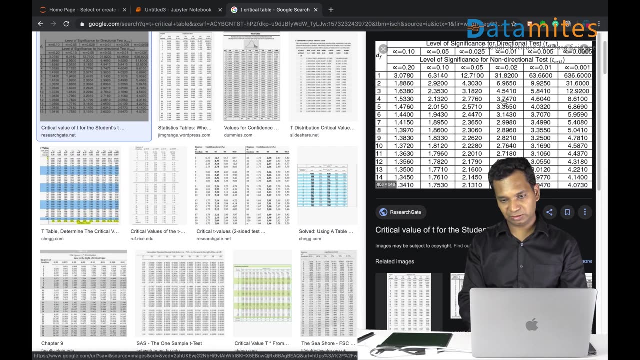 so you don't have to calculate the t critical, you simply so i'm going to google for t critical, t critical table. so t critical table. i can take any one of this. let's say this is t critical. i'm going to open it up as an image. 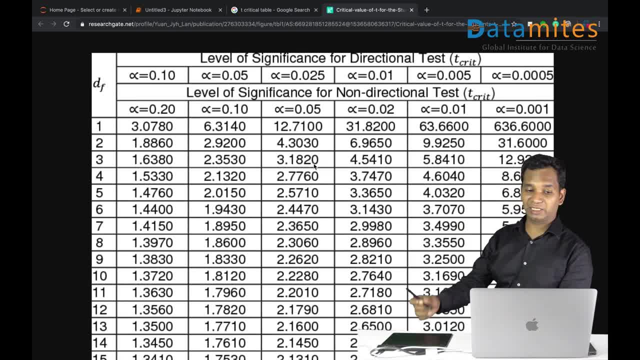 so if you look at here, we have different t critical values of different significance. so i'm looking at this: alpha is equal to 0.05 because we know we are looking at 95 confidence interval, which means five percent alpha five. so this is the test if you're looking for. 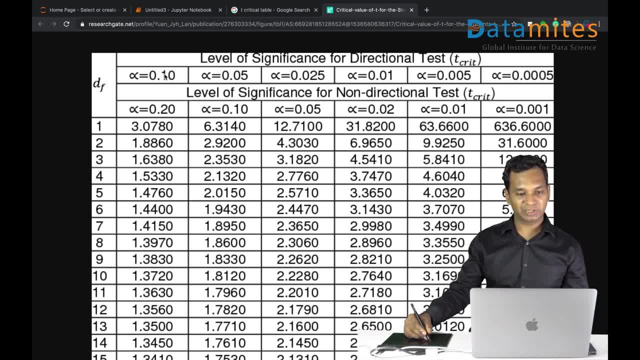 10 percent confidence interval or uh probability 10 percent. come here 90 confidence interval, and this is actually 99 percent confidence interval, which is uh probability is 0.01. so i'm looking at this and these are the degrees of freedom, number of records you have. so we have, i don't know, 12 or. 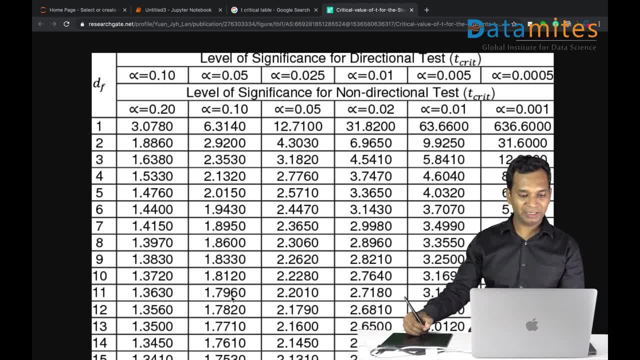 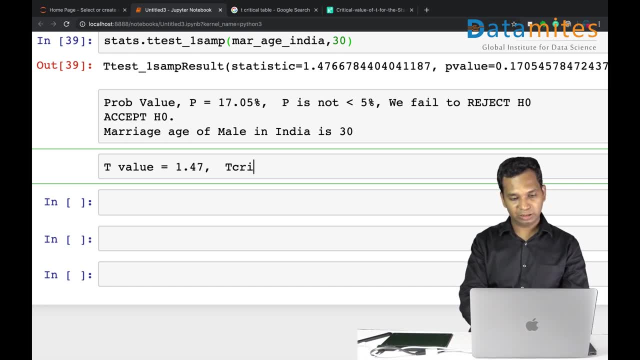 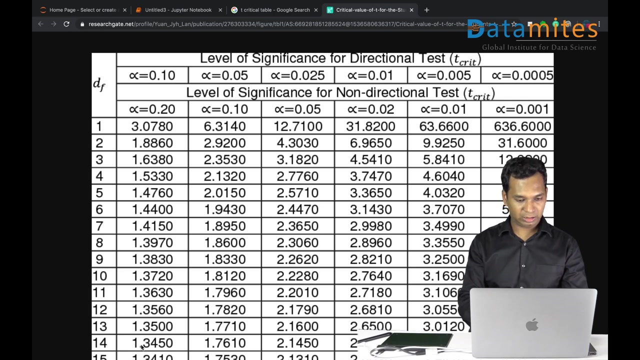 something. so it's coming to 1.79. so from the table i have found, i have found that the t value from the table, my t critical value, critical value or simply tc- i'll just write it down to critical for your simple understanding- is actually 1.79. 1.79- uh, for that i need to know how many records. 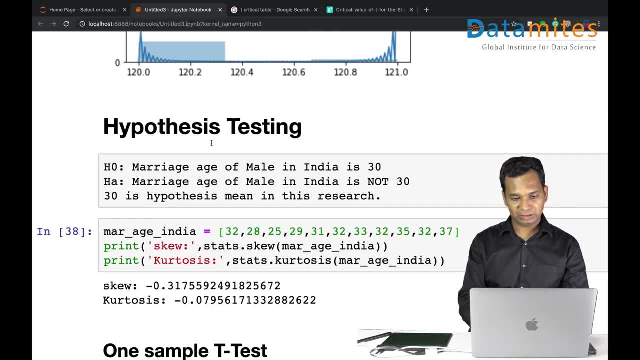 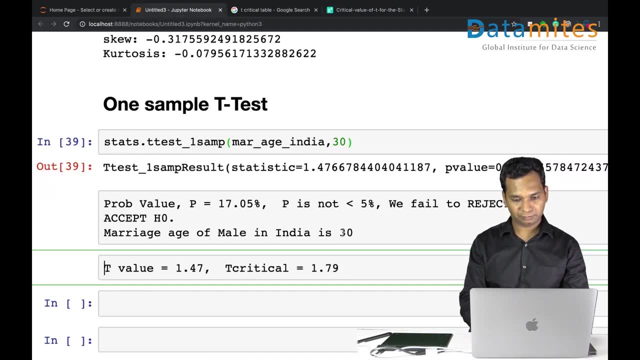 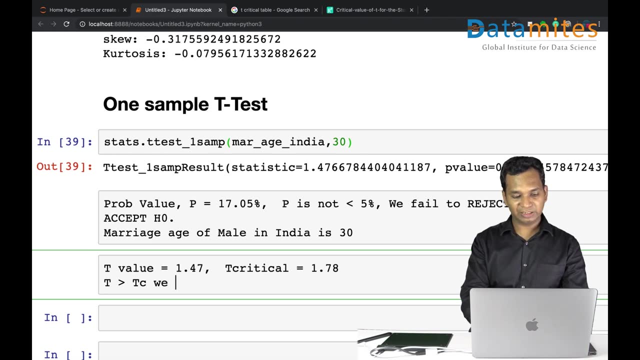 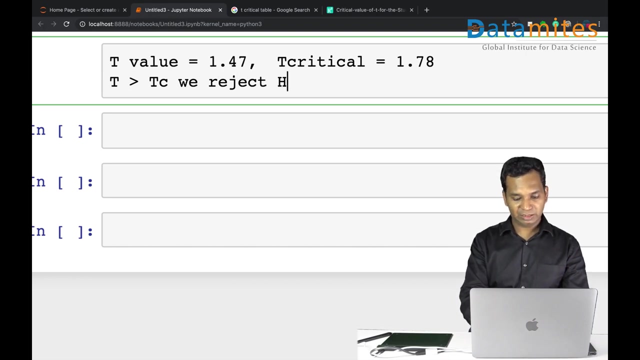 degrees of freedom you have roughly. let's say you have 12. okay, i think it's about 1.78. so what is our principle? if t value is greater than t critical, then we reject. so hope you can see this, where you can reject null hypothesis. is it true here? 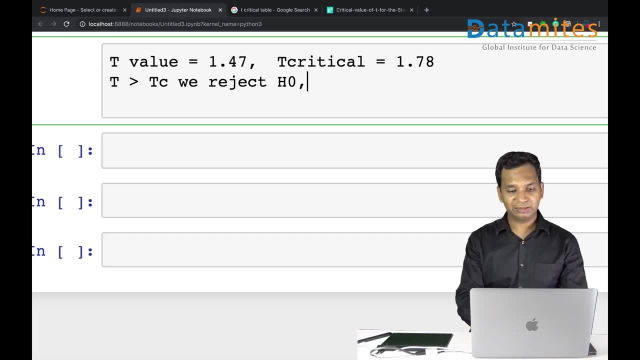 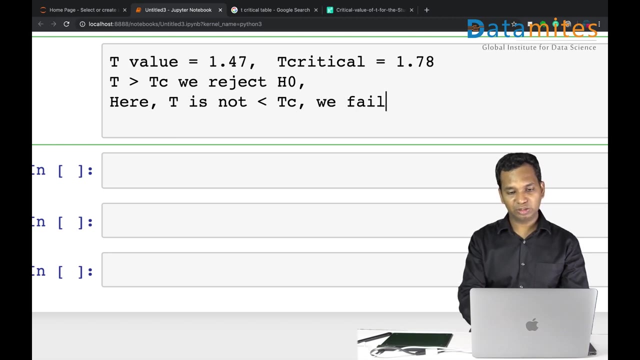 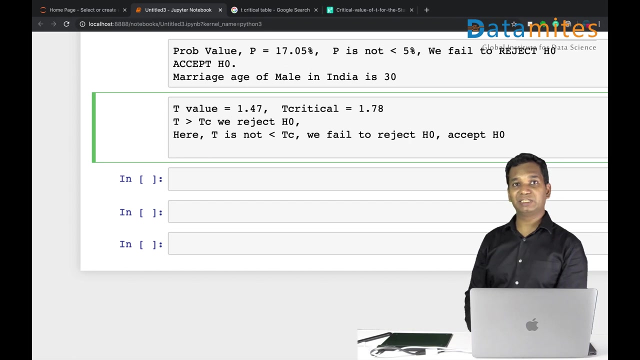 no, your t value is less than t critical, so we fail. so here t value is not, uh, less than t critical model. once again, some calls that here t one. we have tasty here t is not pleasant. so we fail. to reject null hypothesis. so we accept null hypothesis. so the conclusion here is exactly same as the above. 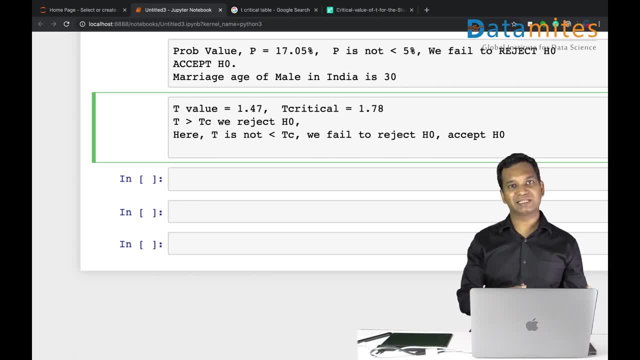 but there we have simply done. did with the p value, which is easily we are obtaining from our python. calculate with the tools- even you have spss or many other r related packages- simply calculate p value. you can do it. but if you want to go with a traditional method, we go with finding the t. 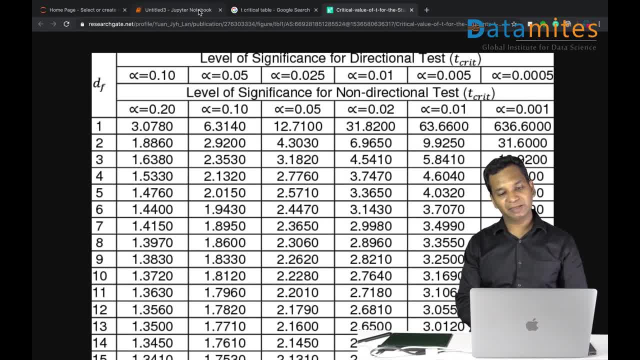 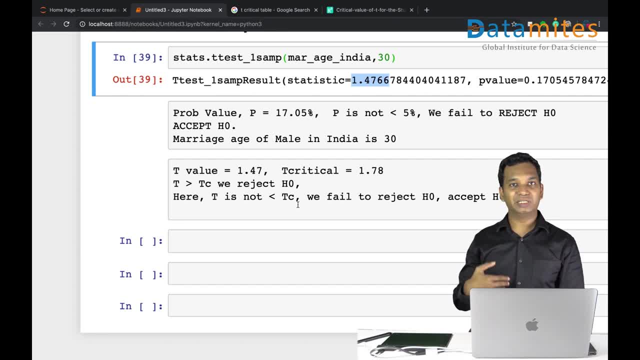 critical from a lookup table- we have a lookup table over here- and then compare the t value which you're getting from the test here with that. if the t value is greater than t critical, then we reject the null hypothesis. if not, we fail to reject the null hypothesis. 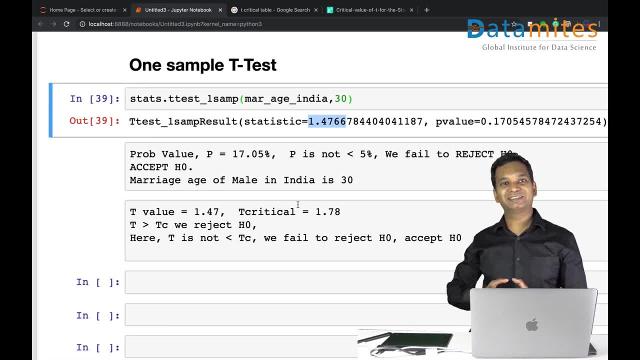 so this is the result of the test. okay, first time when you look at it, it looks a bit of twisting, but please look at the video one more time and you should be able to understand it. it's not very complex, it's actually simple, but it requires a couple of revisions before you understand it. 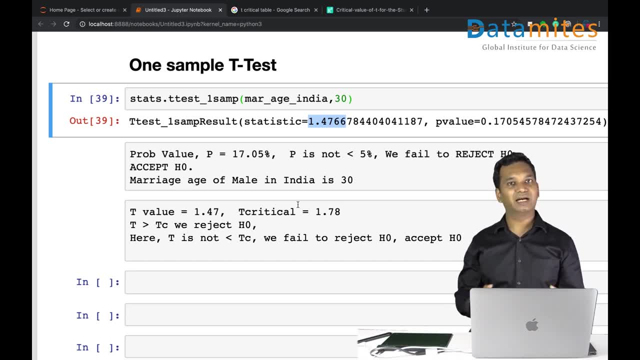 but once you get the logic of hypothesis testing, the further analysis of the further study of other hypothesis testing methods will be will be very easy. um, you like this video. in the next video we are going to talk about two sample independent t test. that's going to be the next video. like the video? please subscribe to the channel. 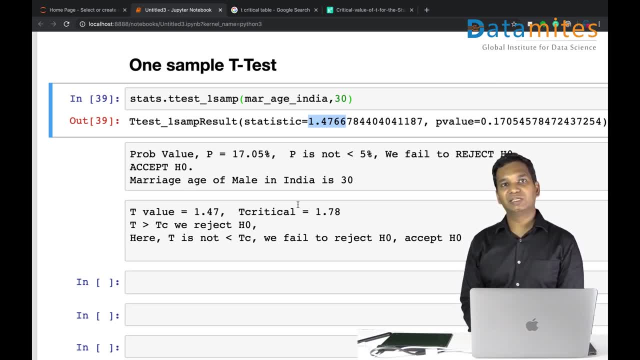 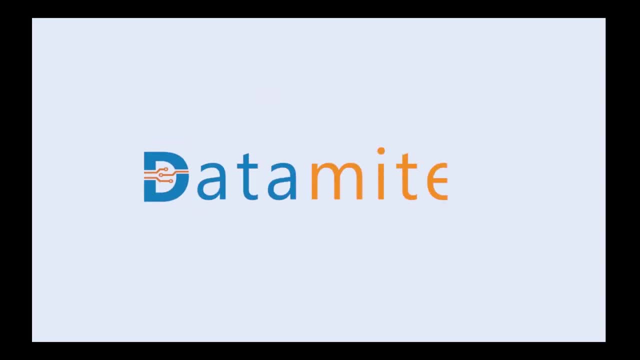 also click the notification button so that when i upload the next video, you will get a notification. thanks for watching. i'll see you in the next video.